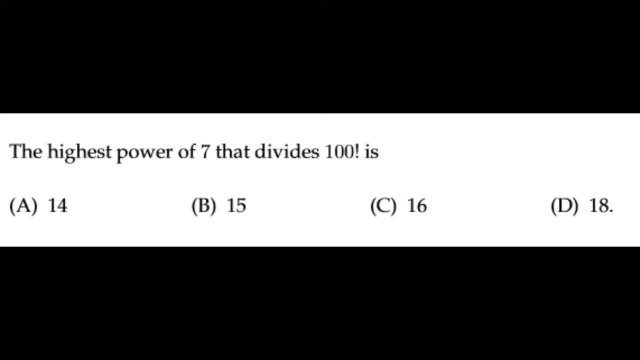 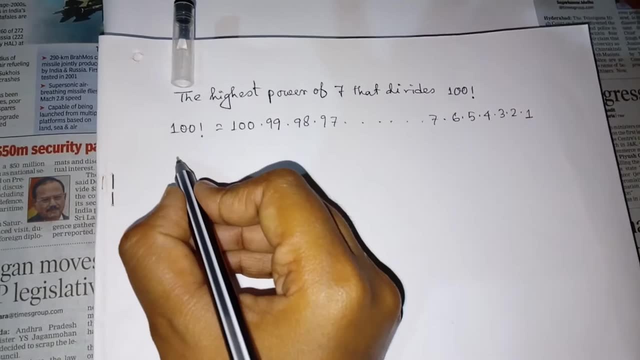 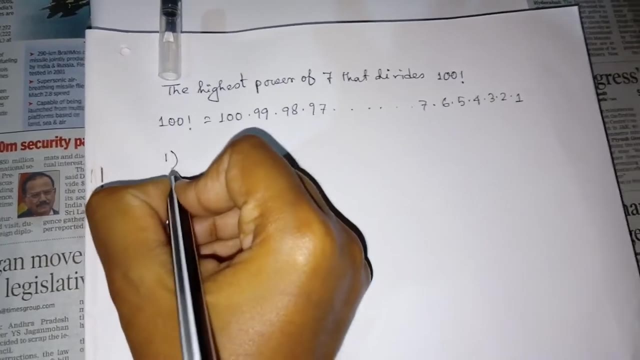 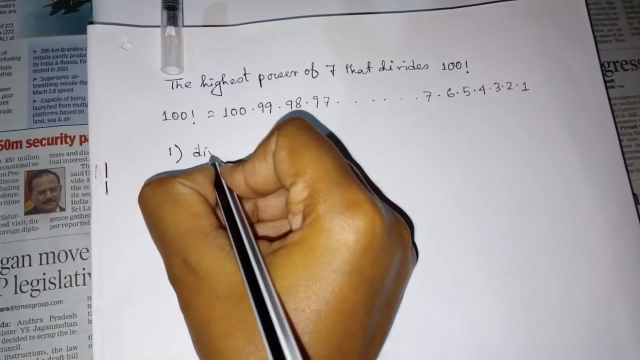 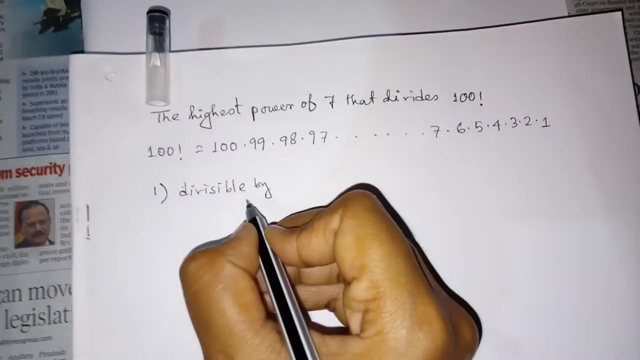 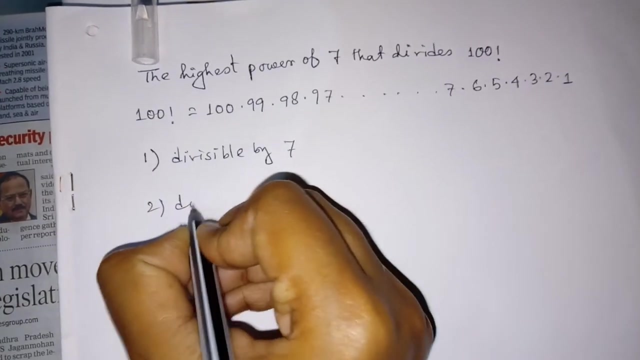 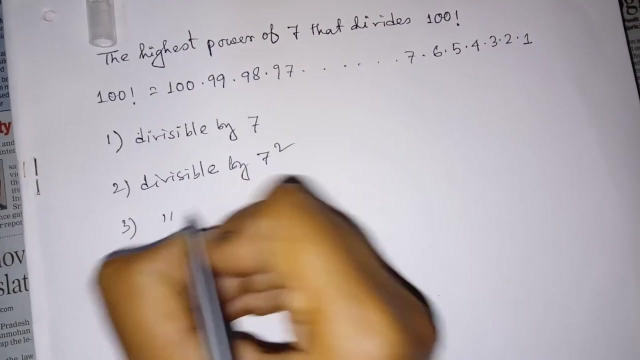 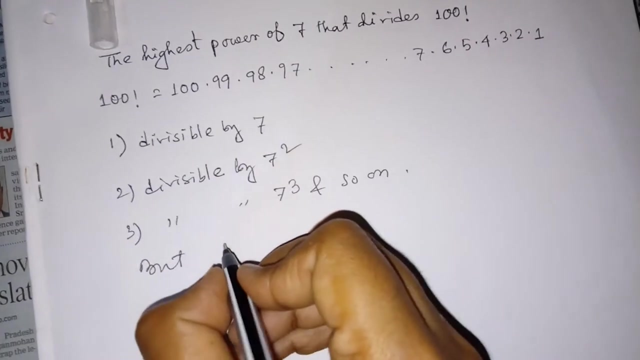 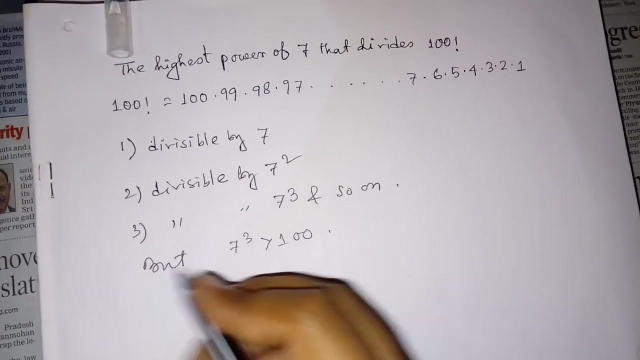 Okay. to do so we have to follow the following rule. First one is numbers which are divisible by, which are divisible by 7.. Second is the vectors which are divisible by 7 square, divisible by 7 cube, and so on, But it is clear that 7 cube greater than 100.. So 3 and further more. 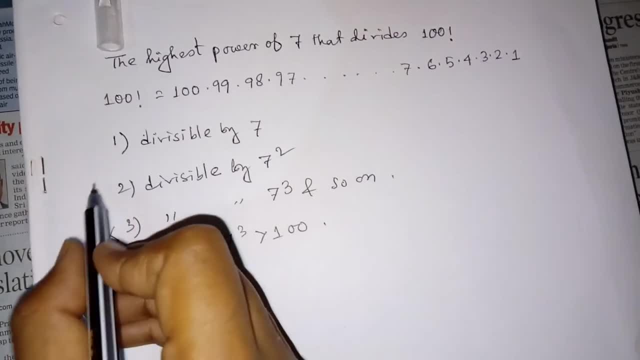 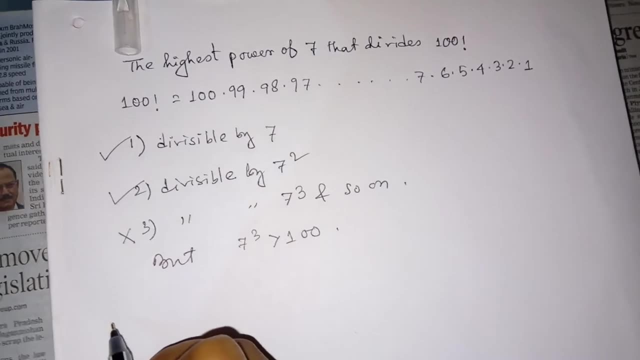 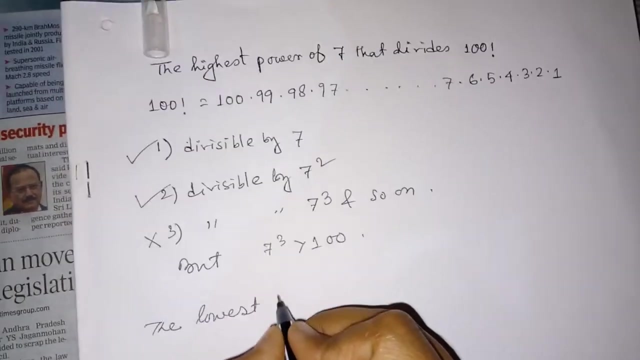 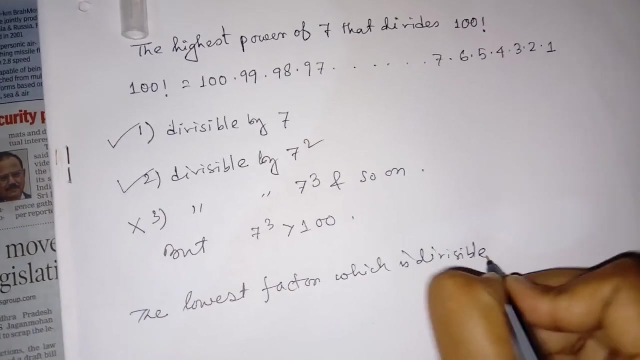 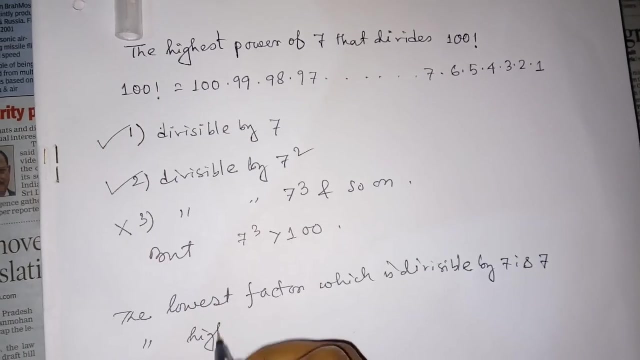 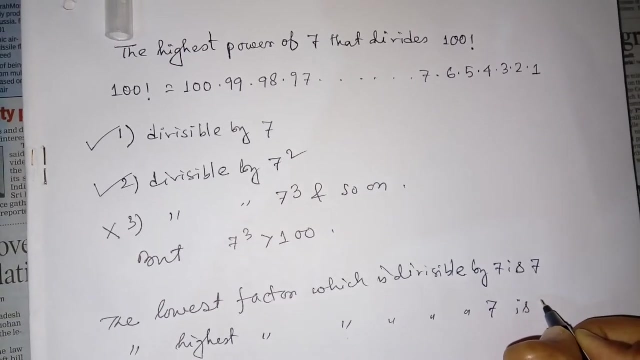 points, not linked it Only. so we have to only find out first two points. Okay, the lowest, the lowest factor which is divisible by divisible by 7 is 7.. And the highest factor which is divisible by 7 is 98.. As 100 is not divisible by 7, it is divisible by 7.. So 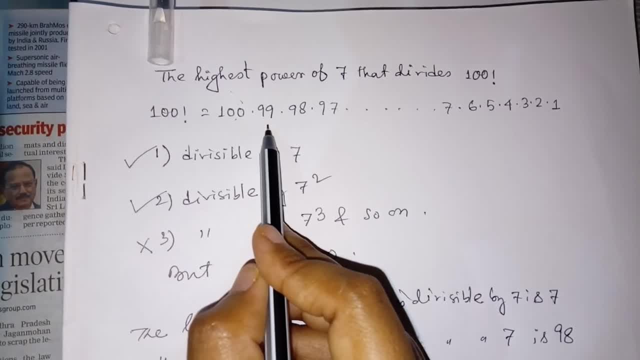 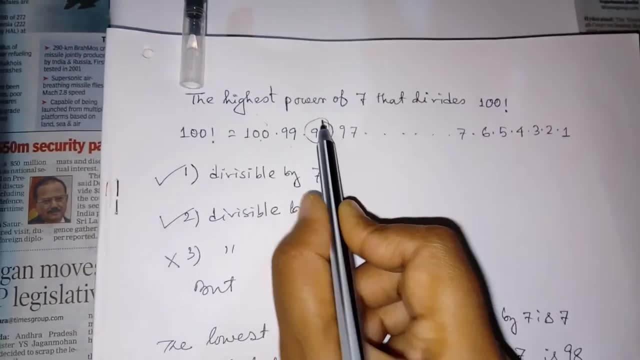 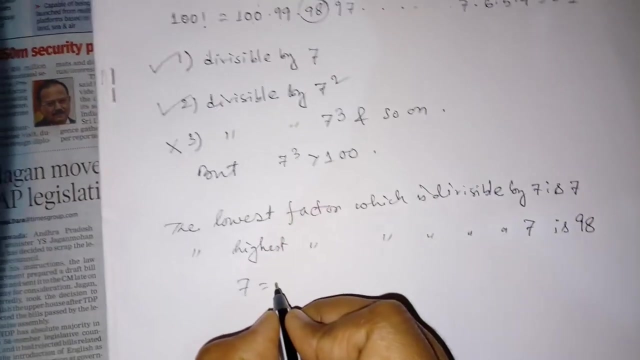 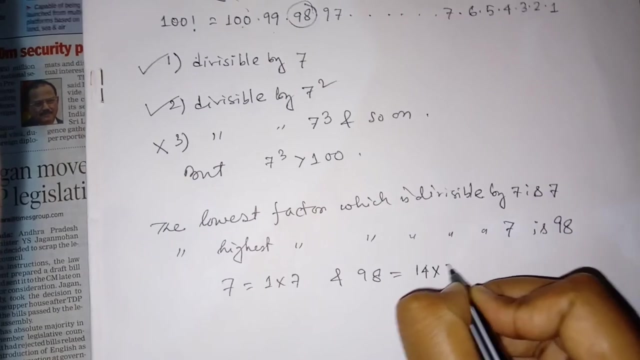 98 is divisible by 7 and 99 also not divisible by 7.. Then 98 is the highest factor which is divisible by 7. Also we can write 7 as 1 into 7 and 98 as 14 into 7.. So we can say: 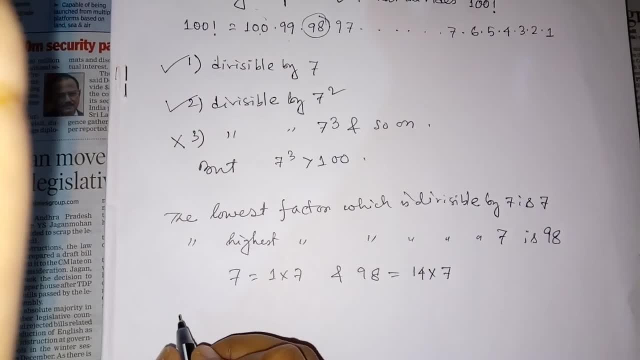 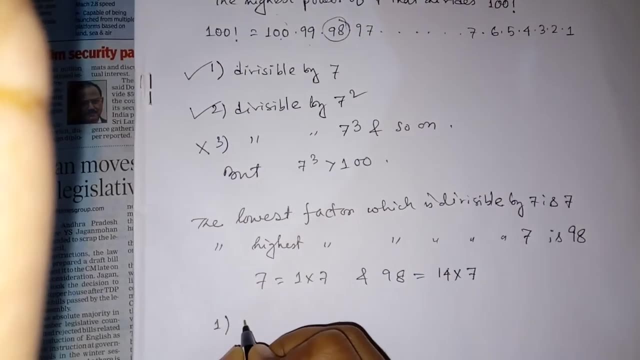 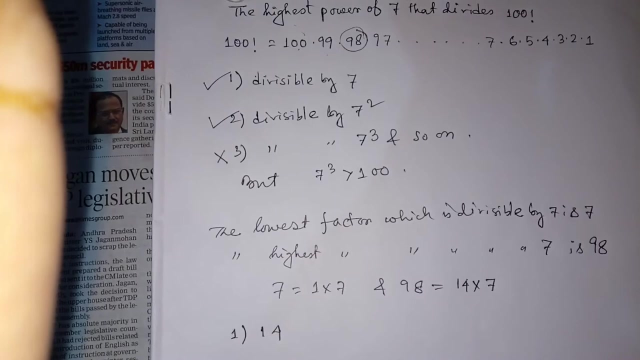 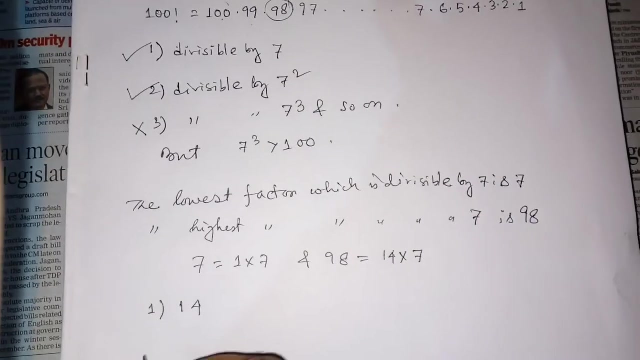 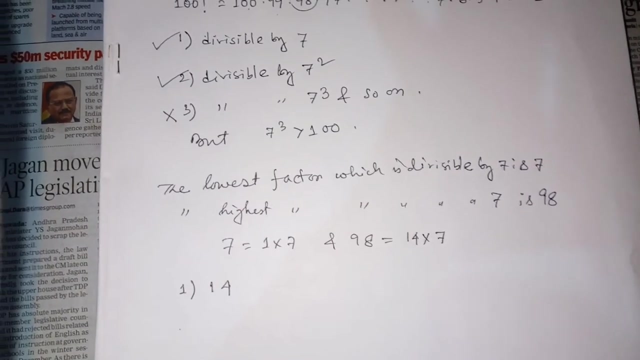 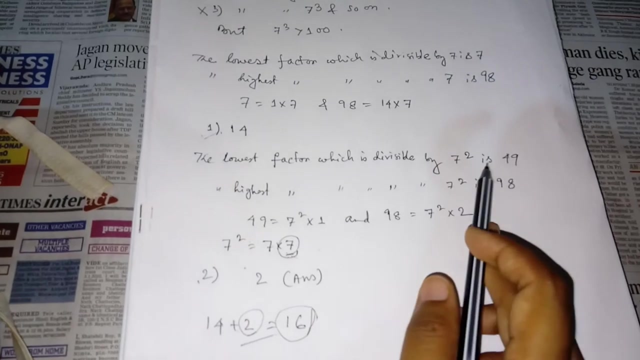 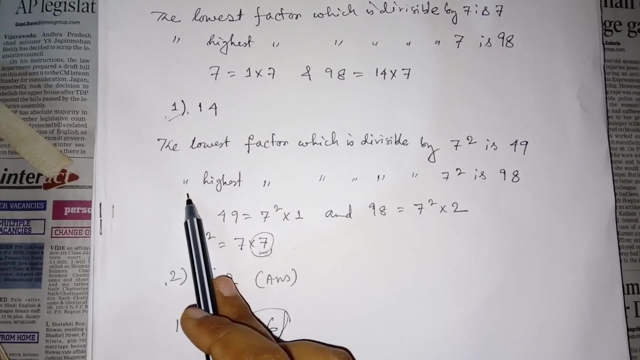 that there are 14 elements, from 7 to 98, which is divisible by 7.. So the answer for first point: it is 14.. Okay, so let us see. Okay, so now let's see. the lowest factor which is divisible by 7 square is 49 and the